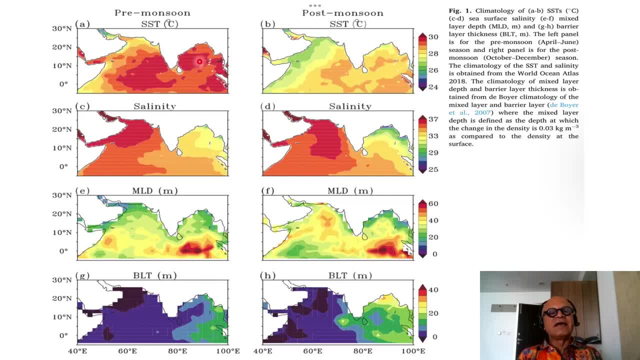 And the Bay of Bengal is not started convecting yet heavily either. So Bay of Bengal remains warm anyways, but you can see during the post-monsoon both of them cool down because the northeasterly winds Begin to pick up. dry continental winds begin to increase the heat loss and associated with these you can see the salinity here. So upwelling brings more salinity and the Arabian Sea is more saline anyways, compared to the Bay of Bengal which has as much freshwater forcing as evaporation- sorry- precipitation and the peaking of the river discharge tends to happen. 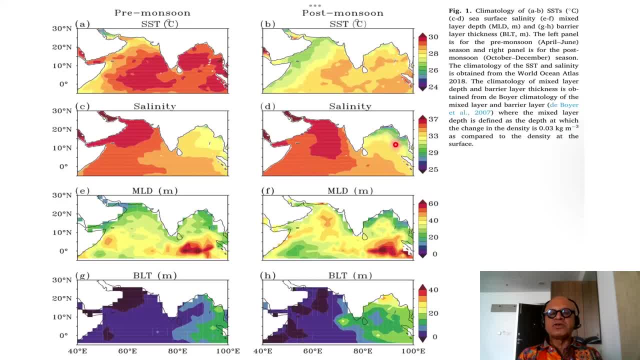 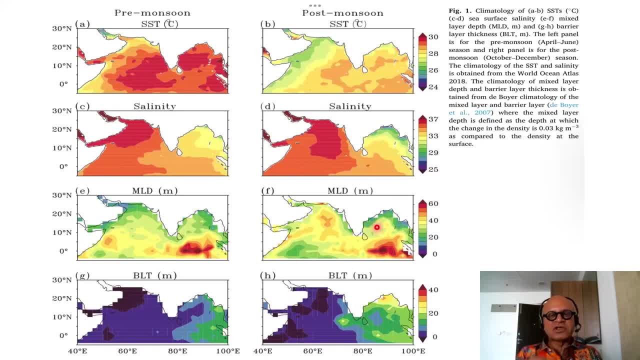 During the post-monsoon season. as you can see, with the reduced salinity here, this leads to some differences in the mixed layer depths as well. But this is a diagnostic study. You have to be careful about how it is defined here. It is defined as a change in the density of 0.03 kilogram per meter cube, So it also doesn't capture the inversions that are happening. 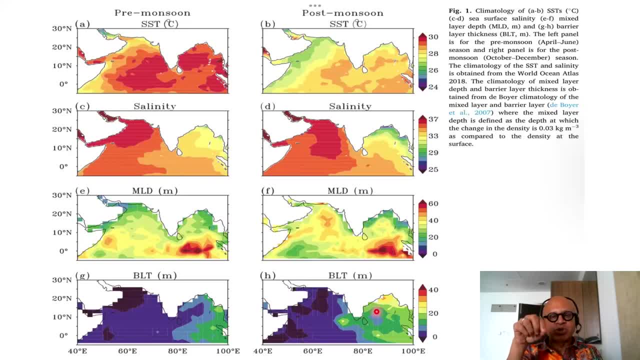 During the post-monsoon season. as you can see, with the reduced salinity here, this leads to some differences in the mixed layer depths as well. But this is a diagnostic study. You have to be careful about how it is defined here. It is defined as a change in the density of 0.03 kilogram per meter cube, So it also doesn't capture the inversions that are happening. 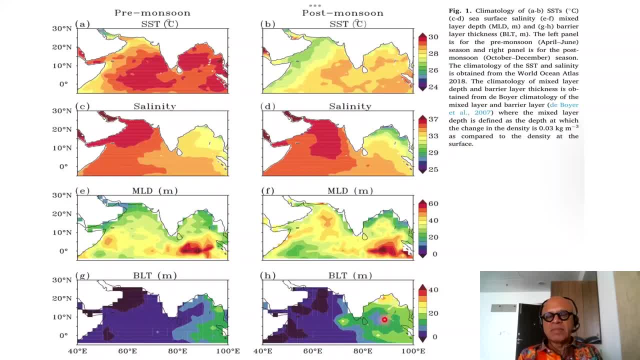 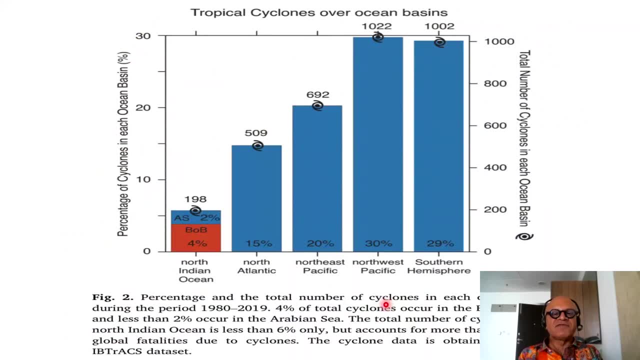 During the post-monsoon season. as you can see, with the reduced salinity here, this leads to some differences in the mixed layer depths as well. But this is a diagnostic study. You have to be careful about how it is defined here. It is defined as a change in the mixed layer depths as well, But this is a diagnostic study. You have to be careful about how it is defined here. It is defined as a change in the mixed layer depths as well, But this is a diagnostic study. You have to be careful about how it is defined here. It is defined as a change in the mixed layer depths as well, But this is a diagnostic study. You have to be careful about how it is defined here. It is defined as a change in the mixed layer depths as well, But this is a diagnostic study. You have to be careful about how it is defined here. It is defined as a change in the mixed layer depths as well, But this is a diagnostic study. You have to be careful about how it is defined here. It is defined as a specific, gets even more typhoons, cyclones, but Northwest Pacific is the most active in terms of producing about 30% of the total number of cyclones. whereas Arabian Sea has 2% and Bay of Bengal has 4%, Southern Hemisphere as a whole has only 29% and is less than just the Northwest Pacific. 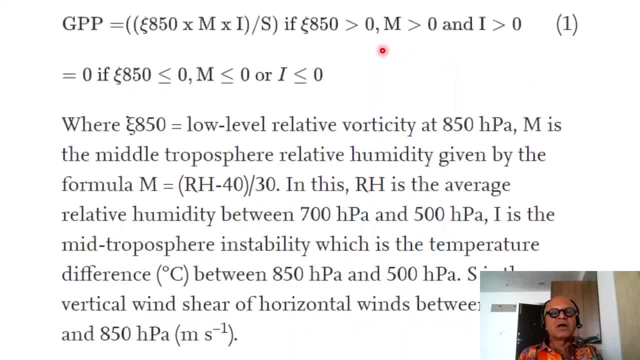 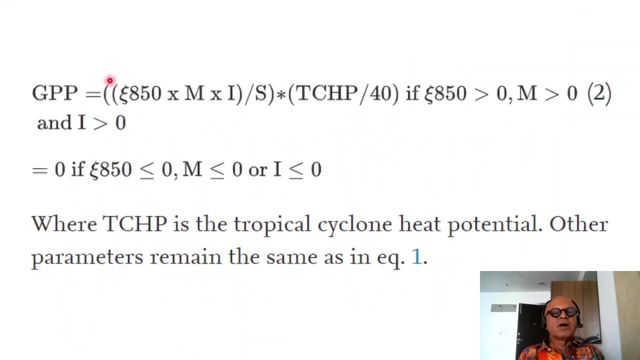 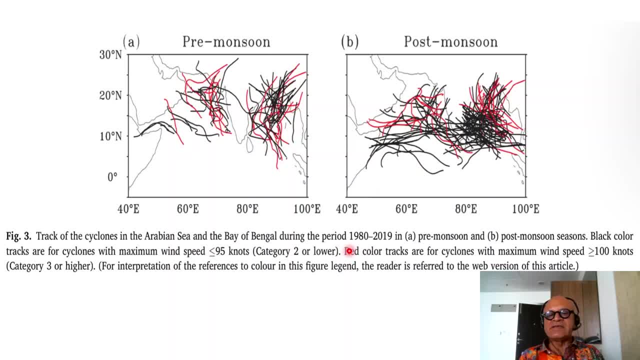 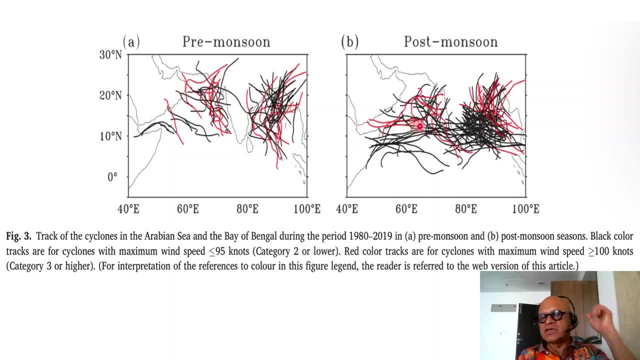 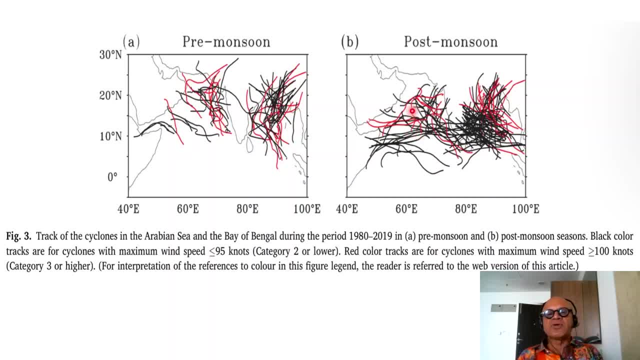 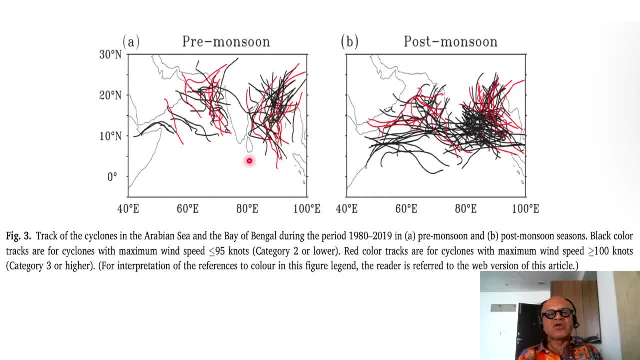 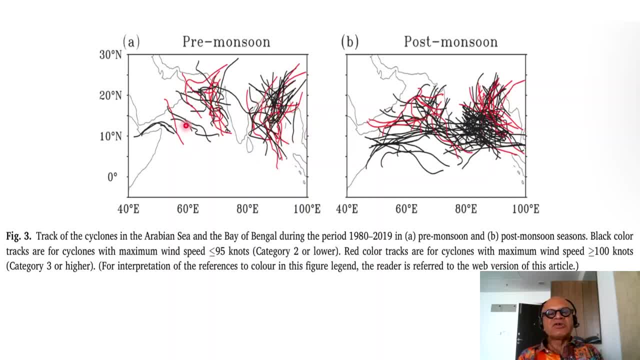 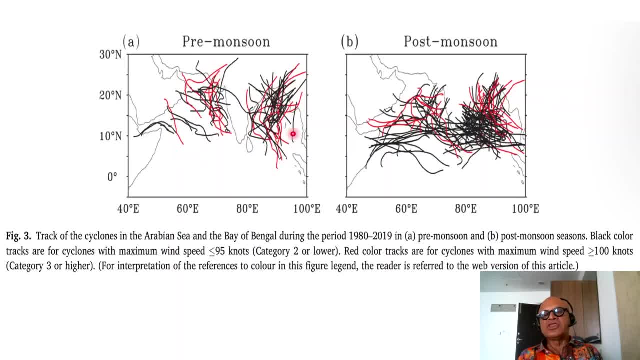 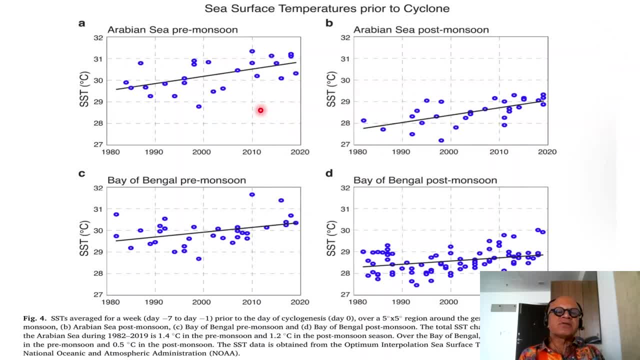 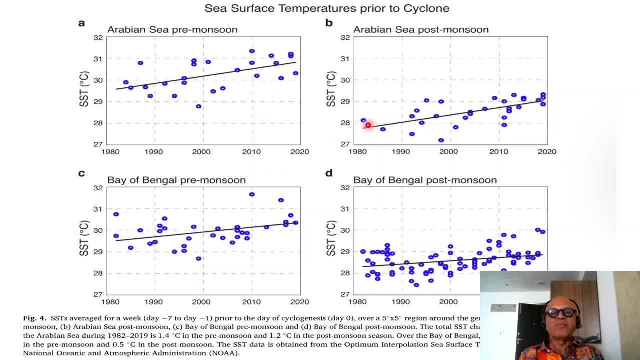 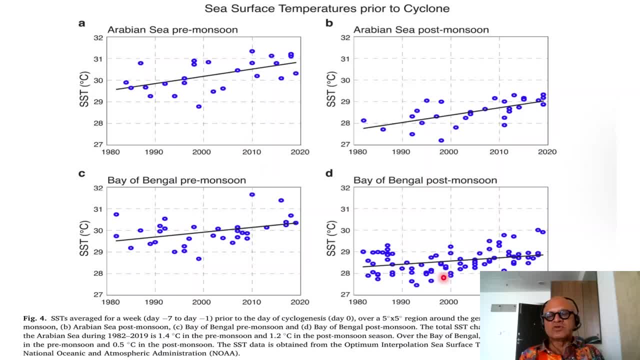 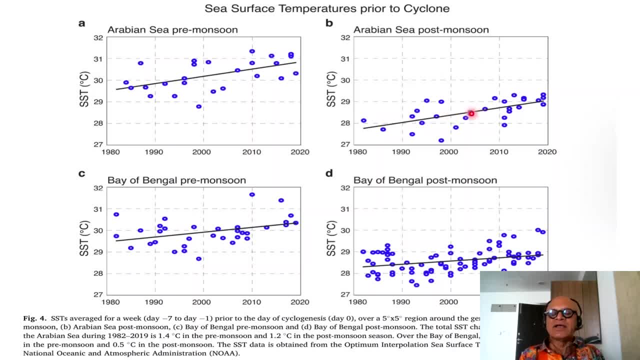 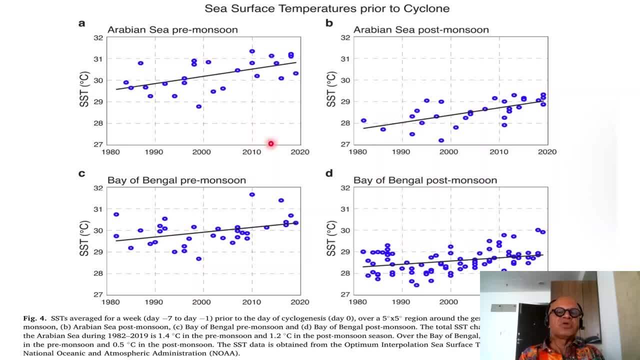 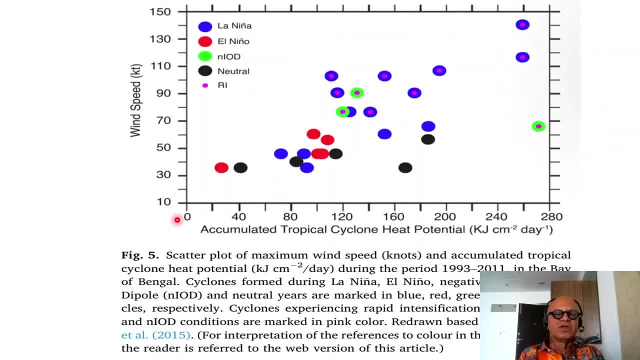 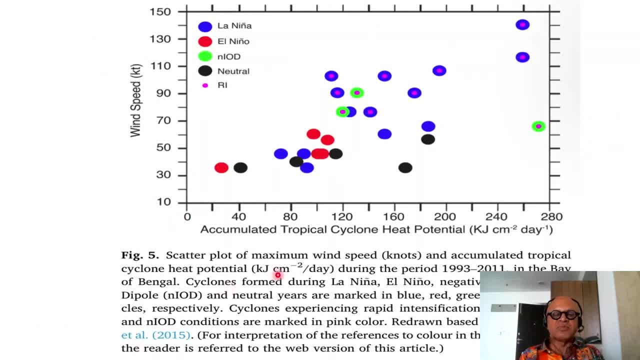 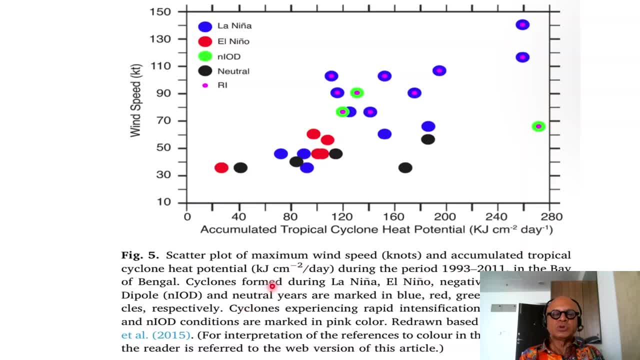 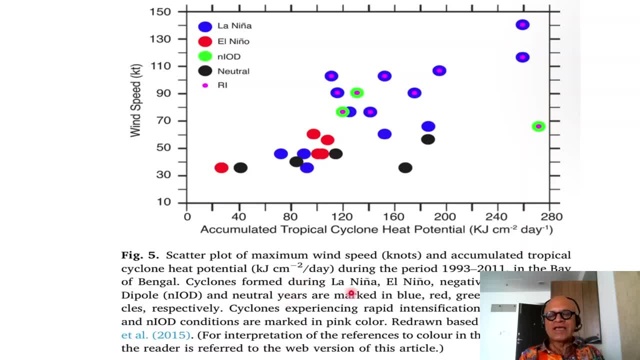 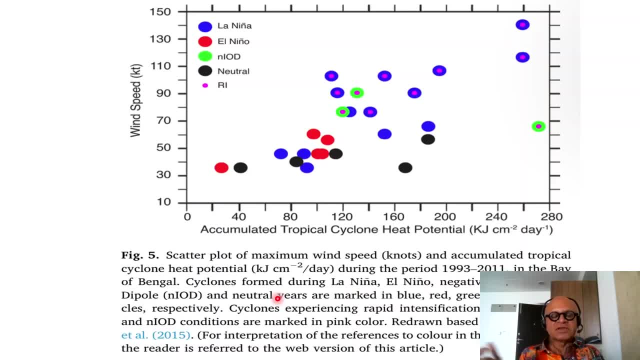 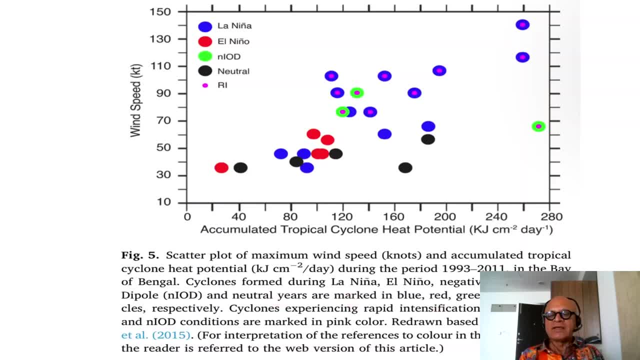 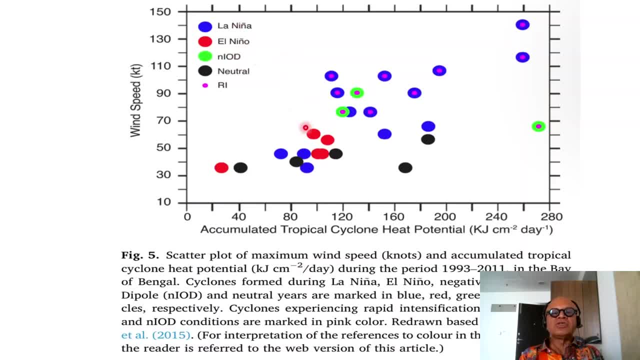 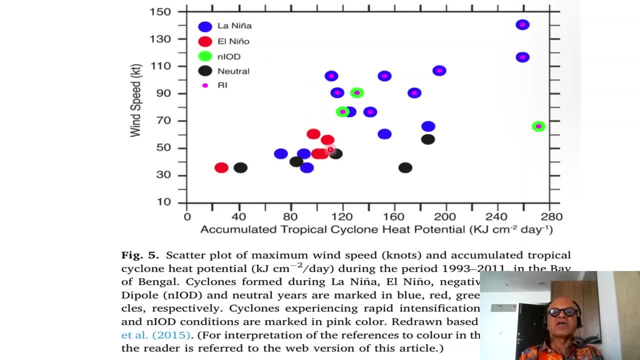 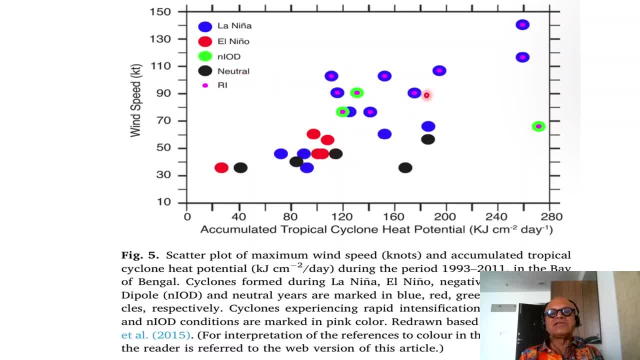 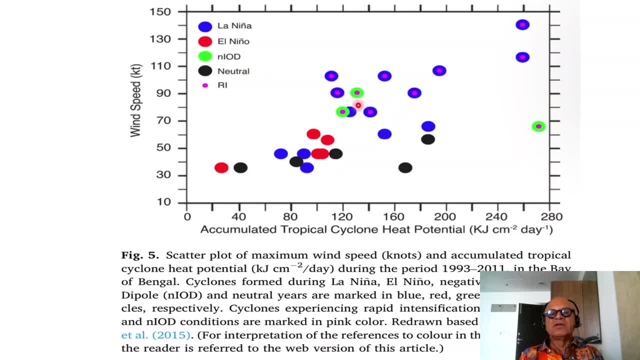 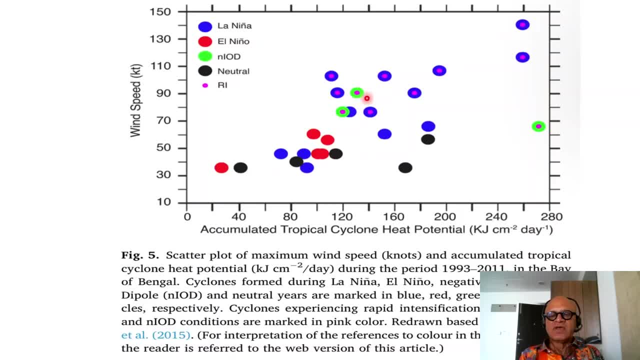 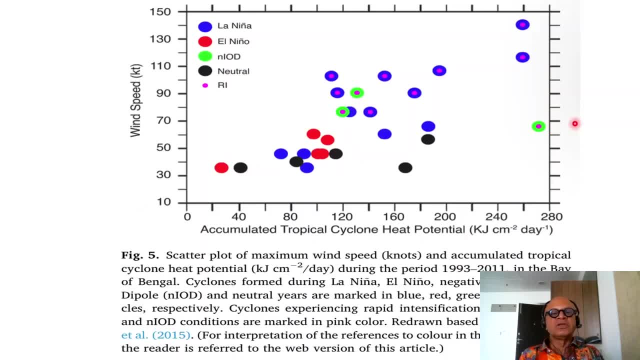 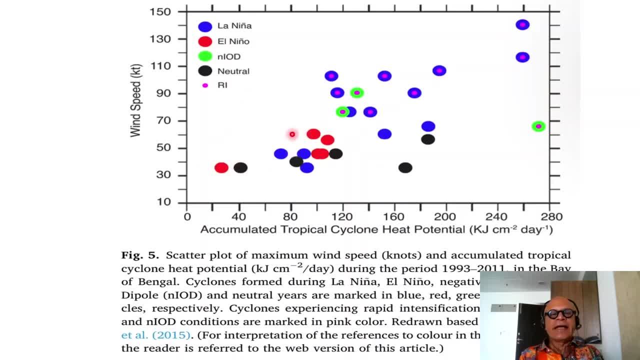 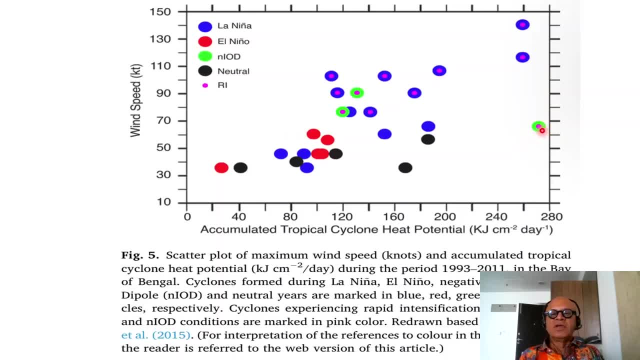 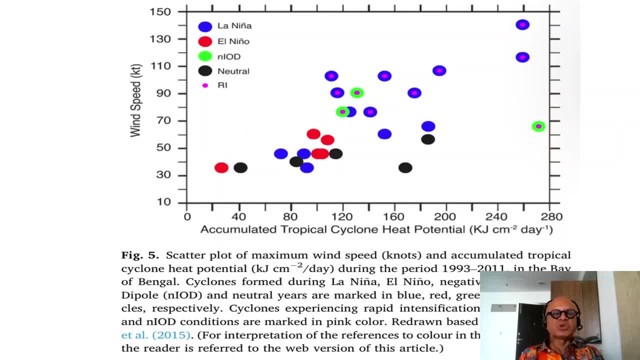 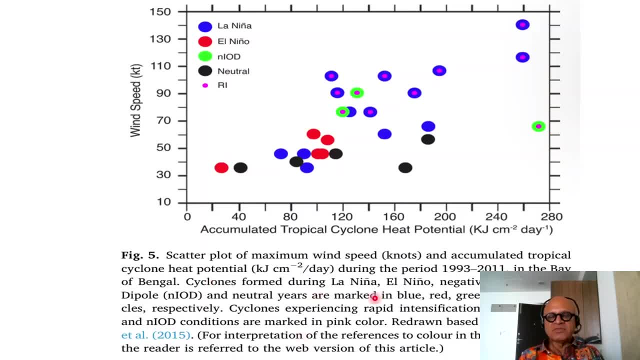 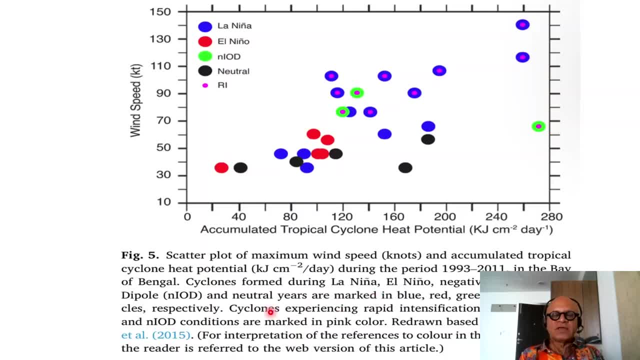 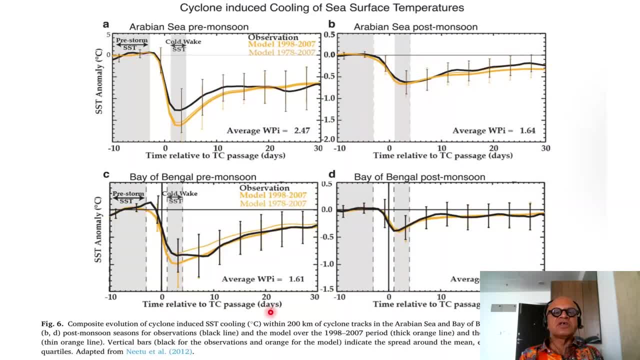 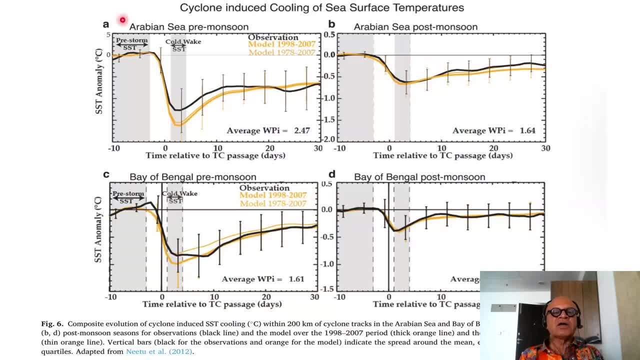 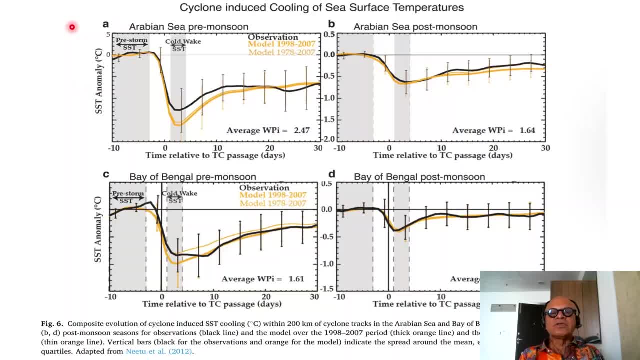 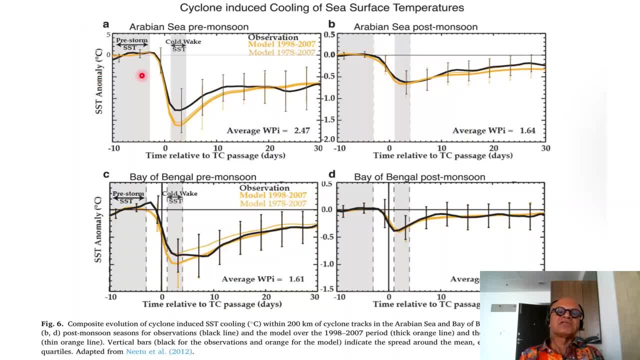 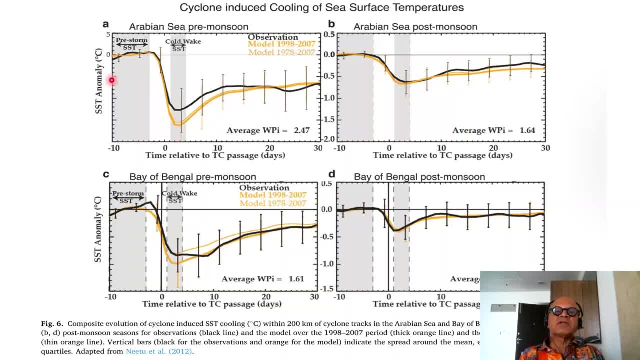 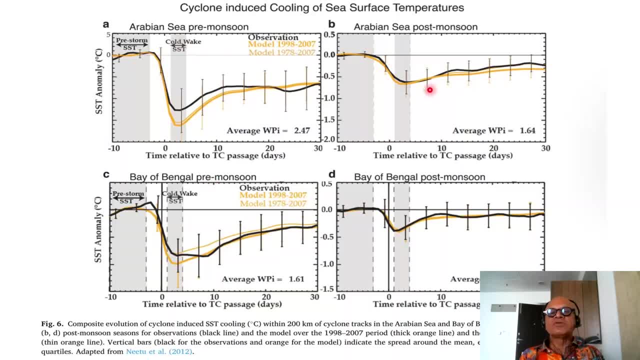 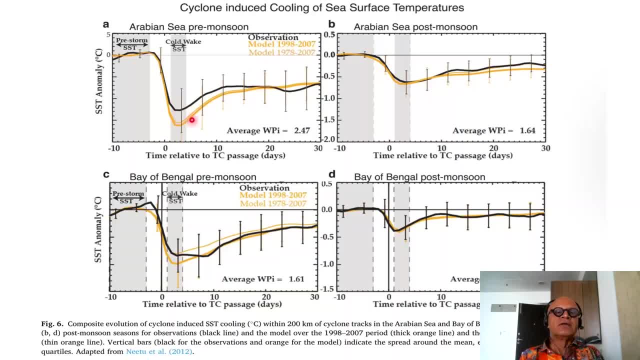 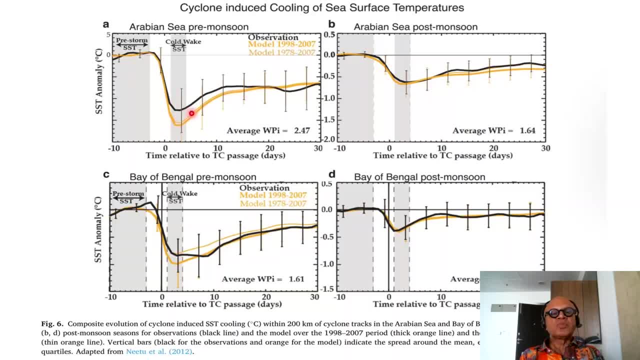 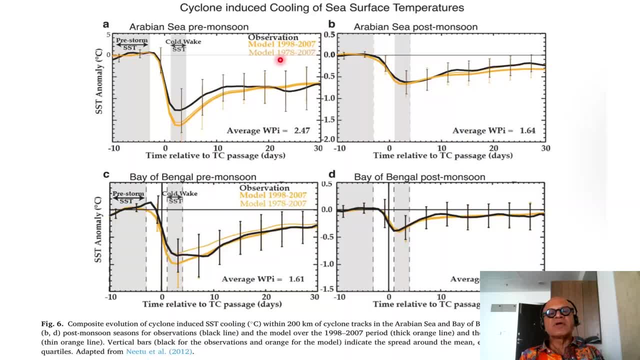 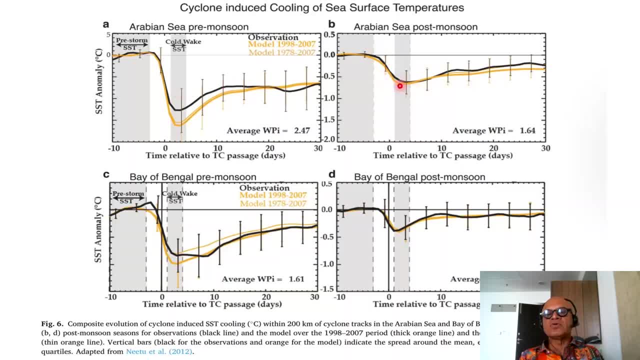 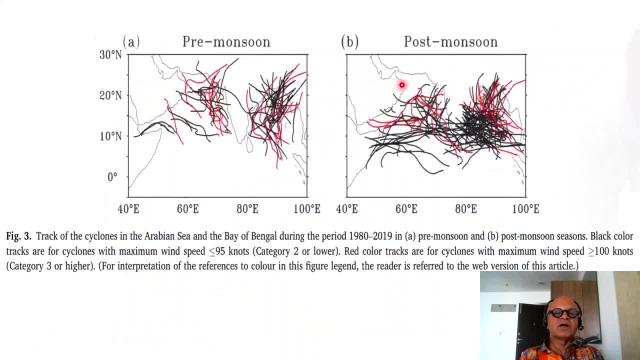 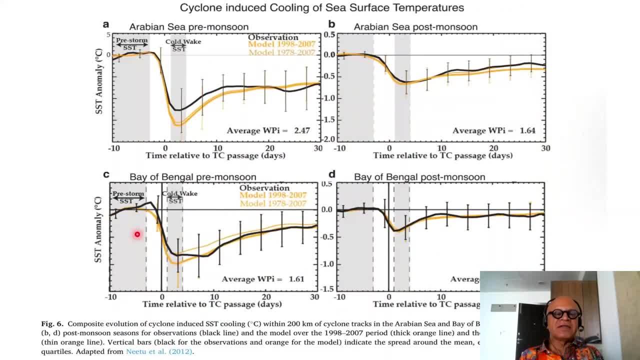 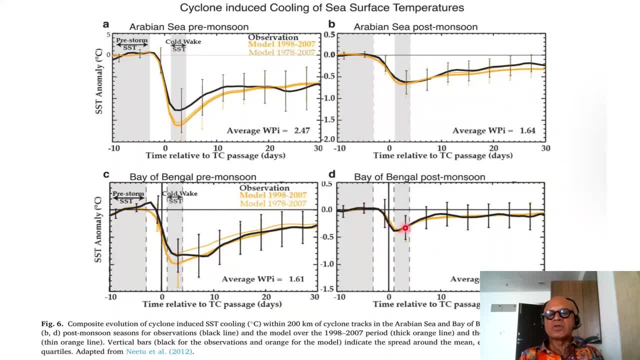 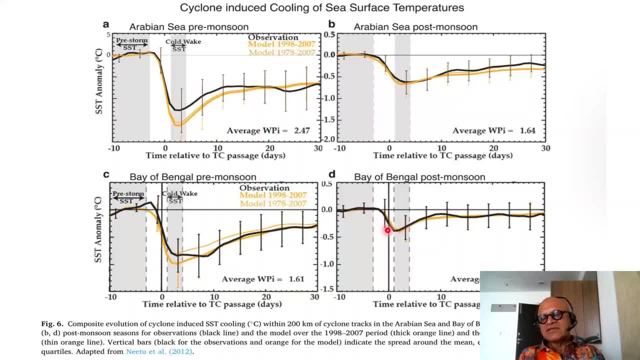 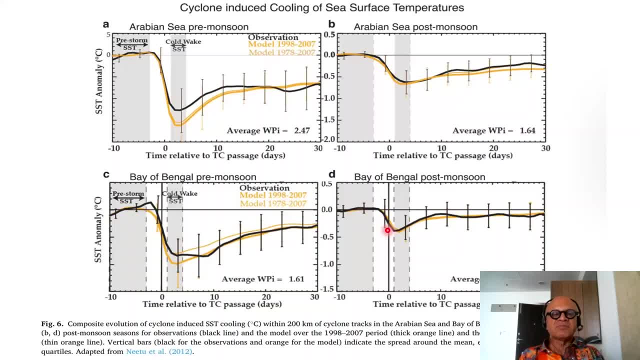 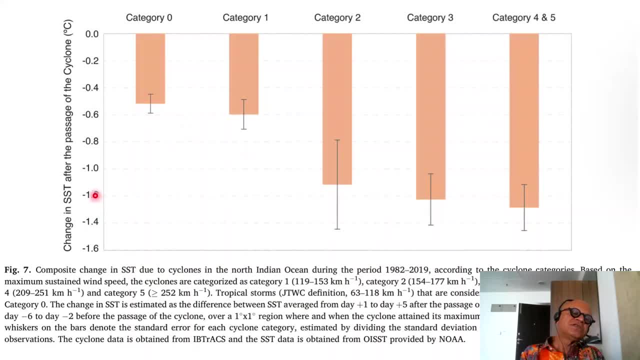 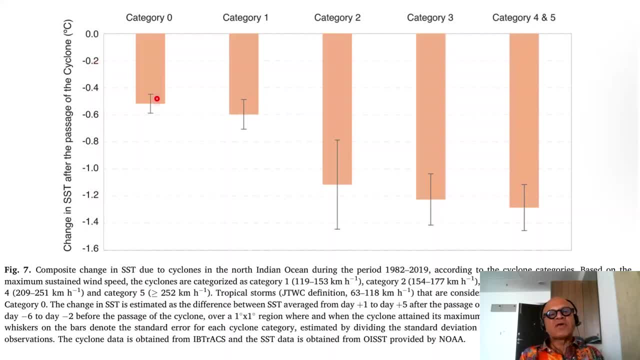 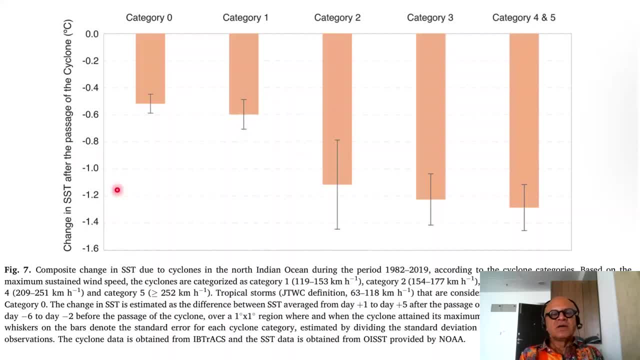 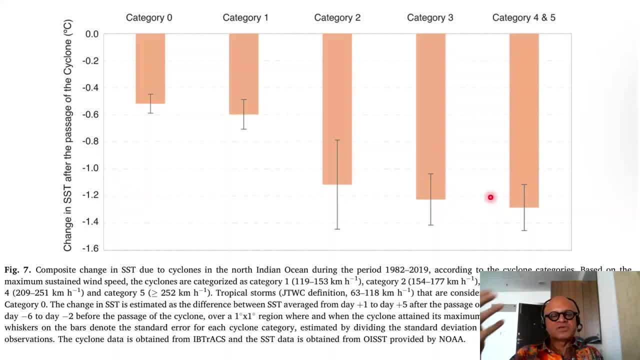 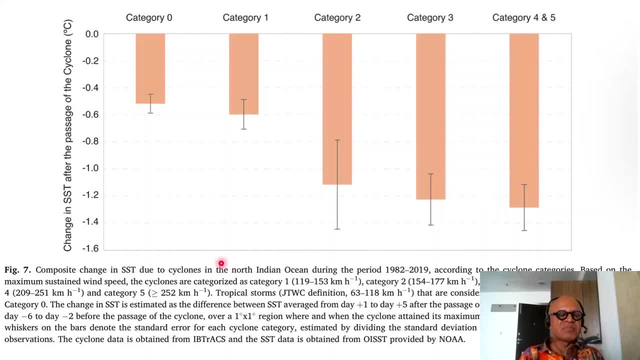 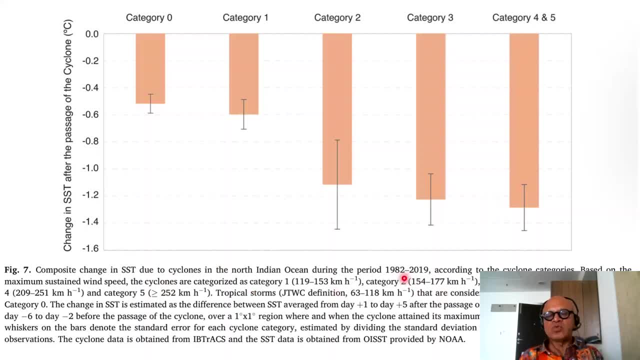 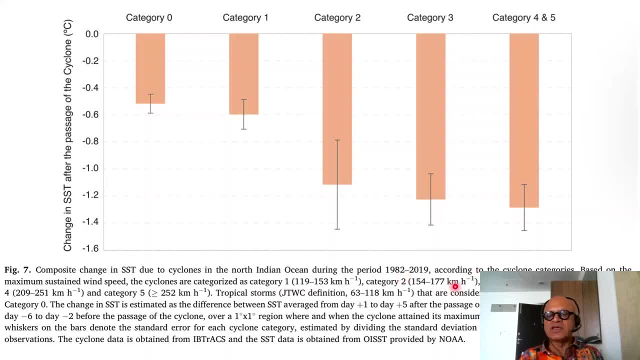 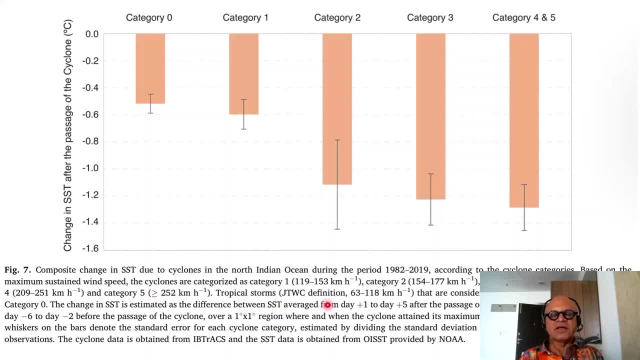 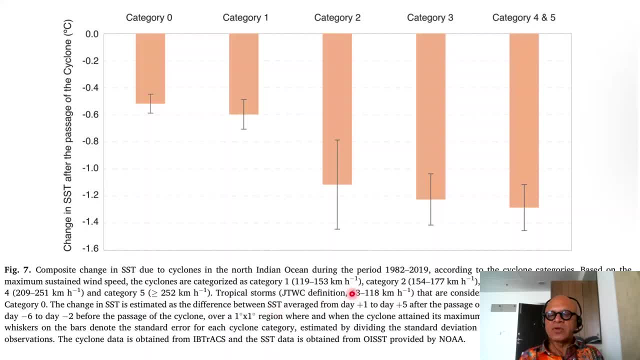 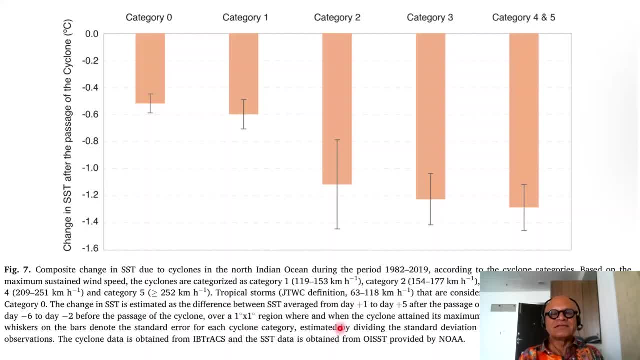 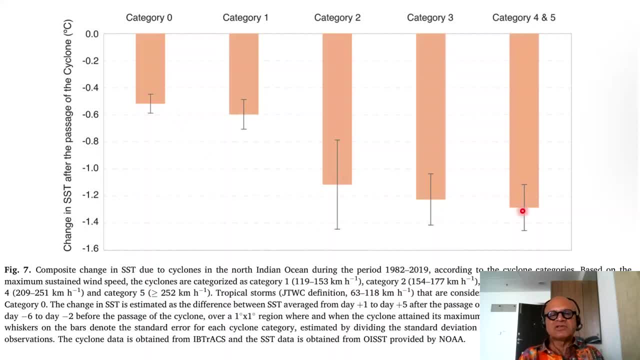 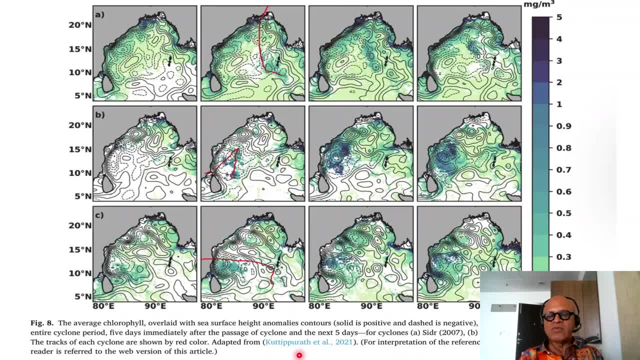 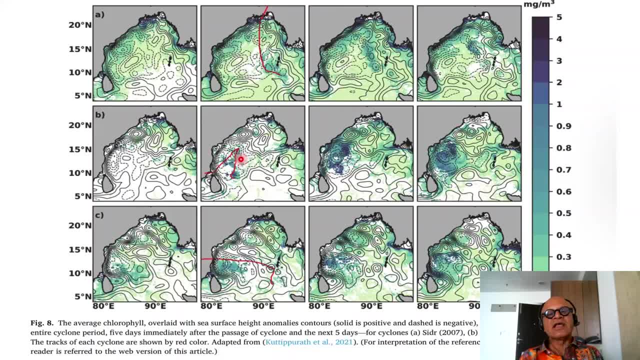 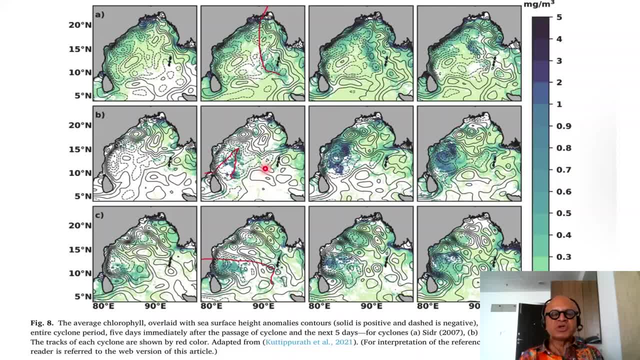 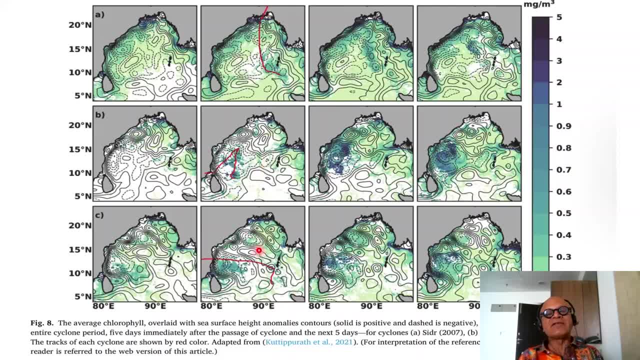 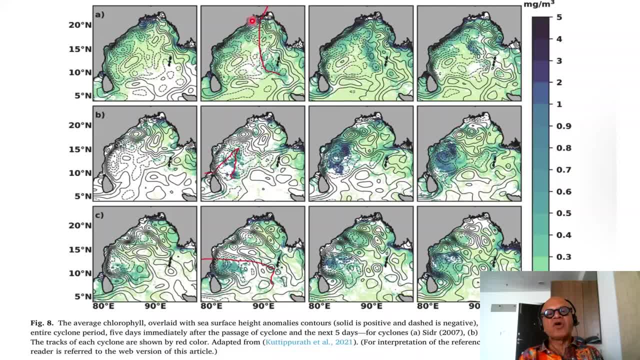 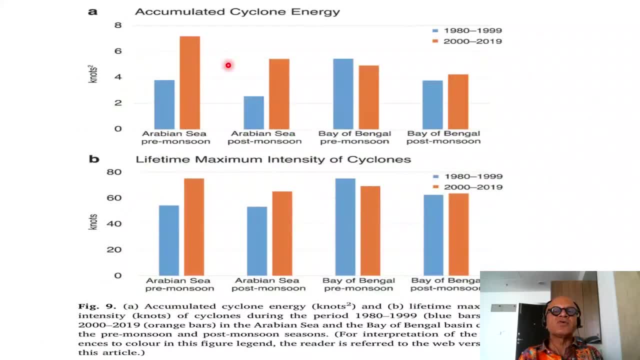 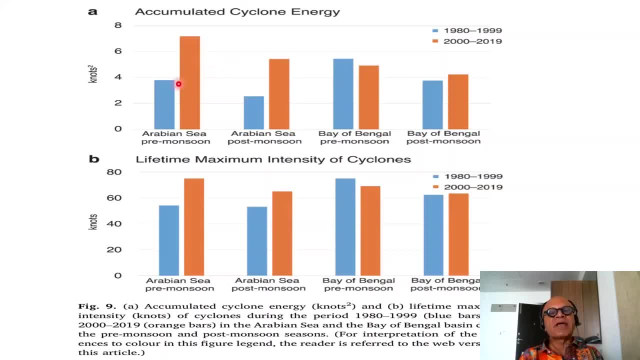 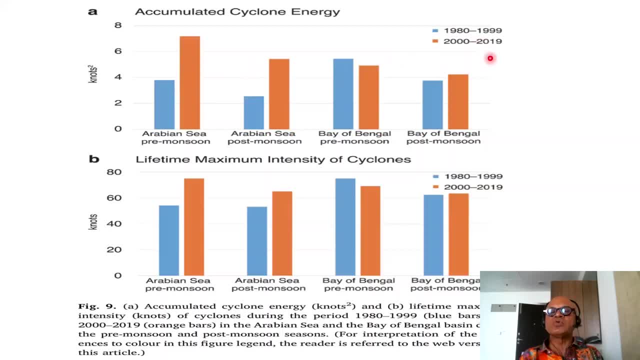 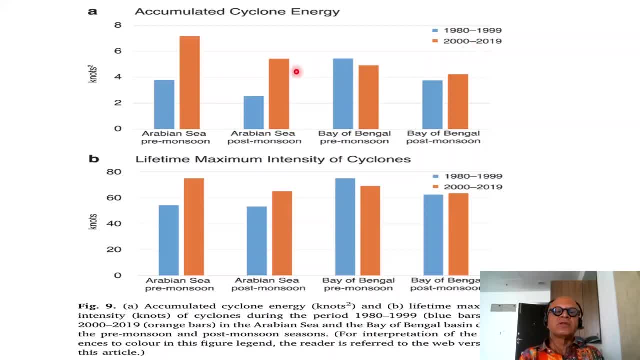 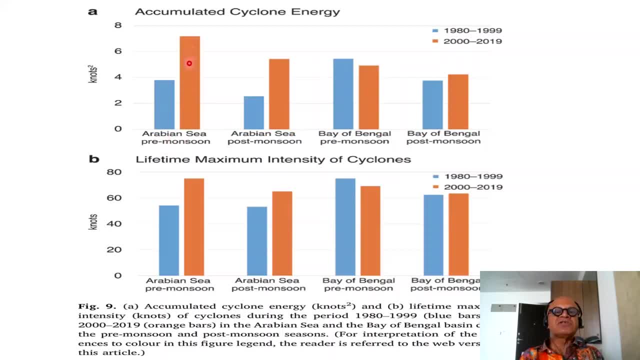 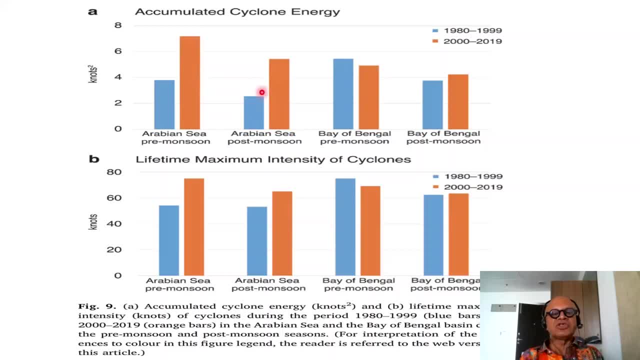 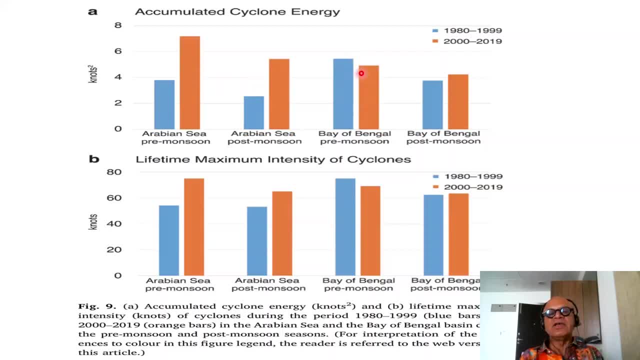 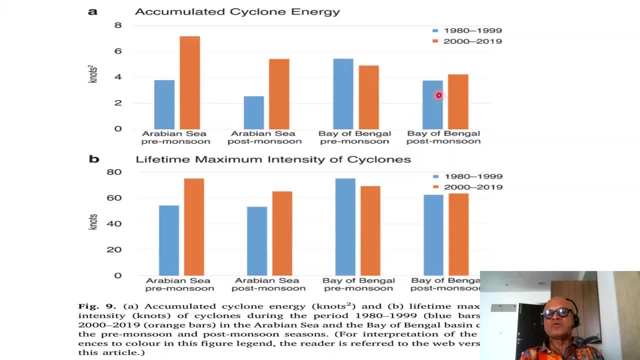 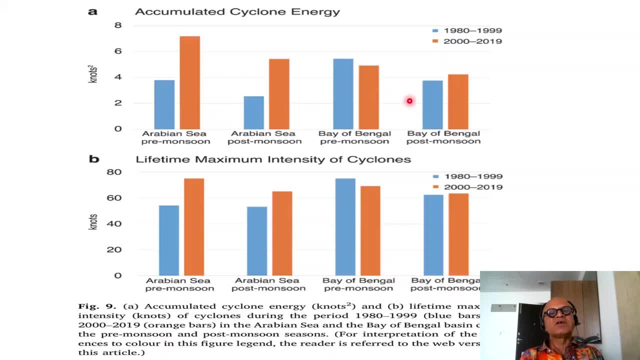 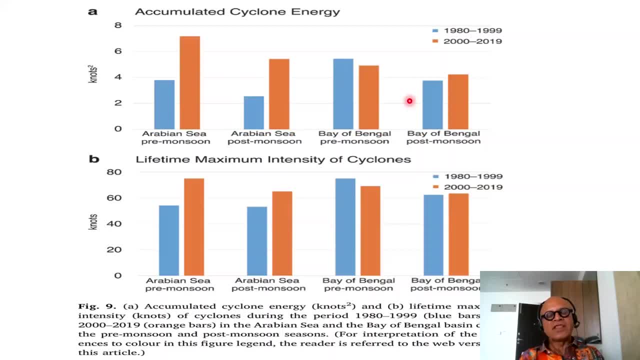 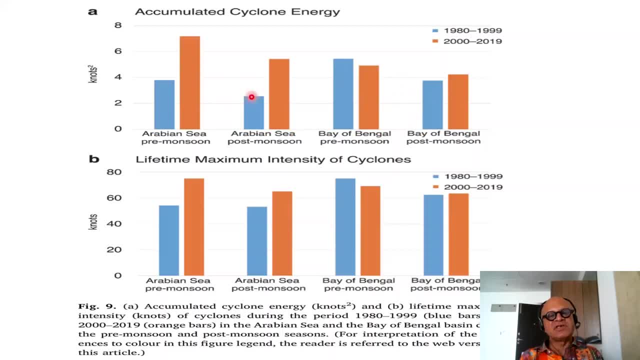 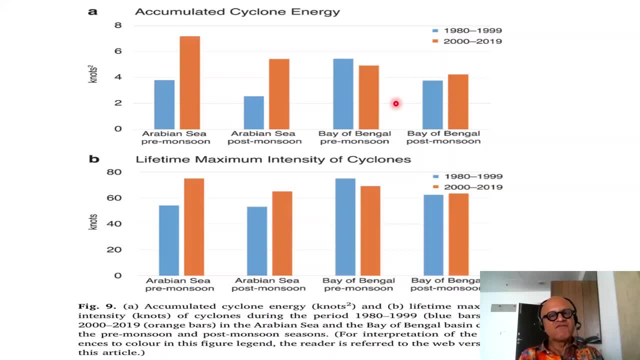 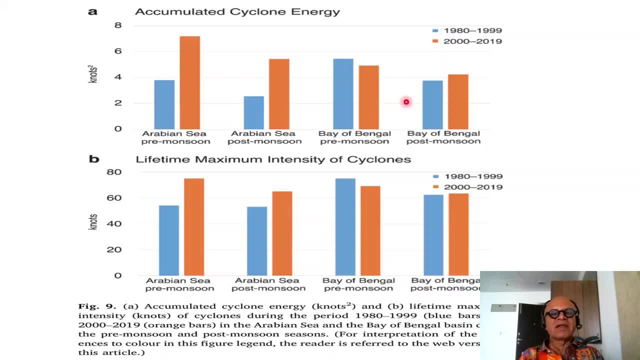 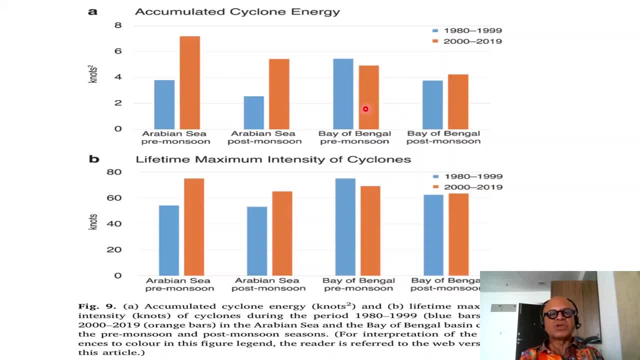 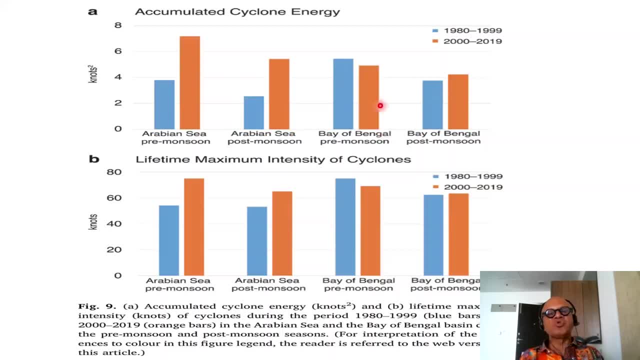 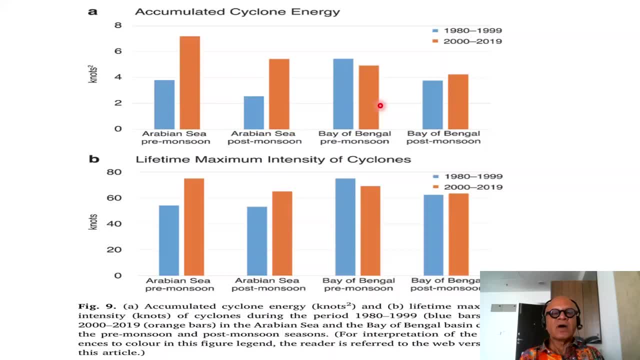 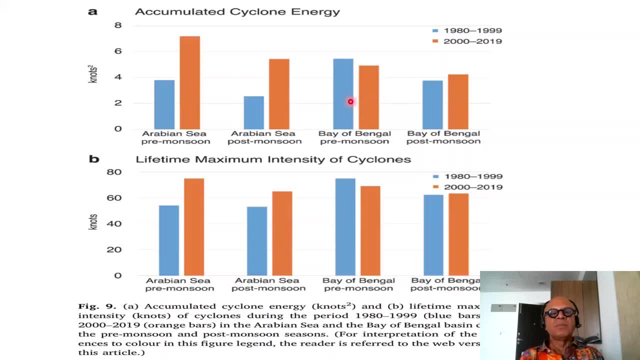 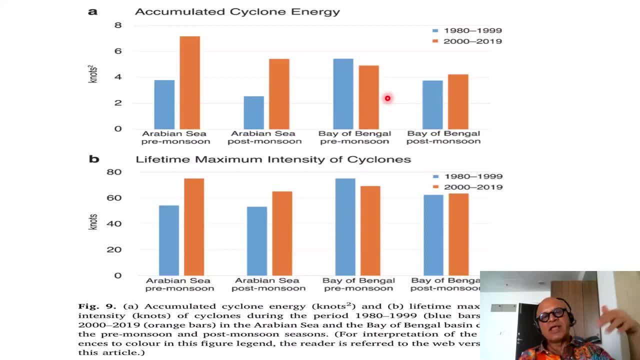 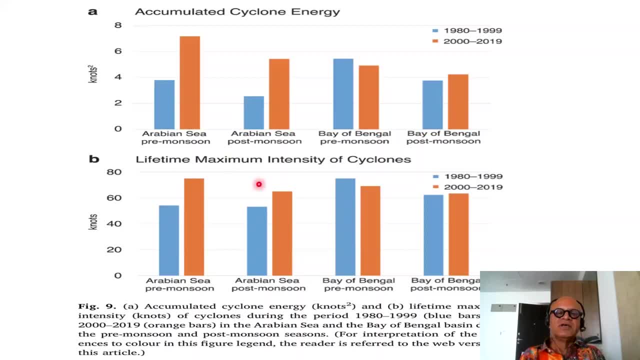 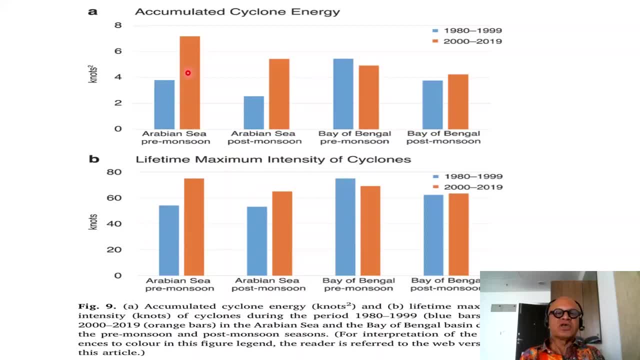 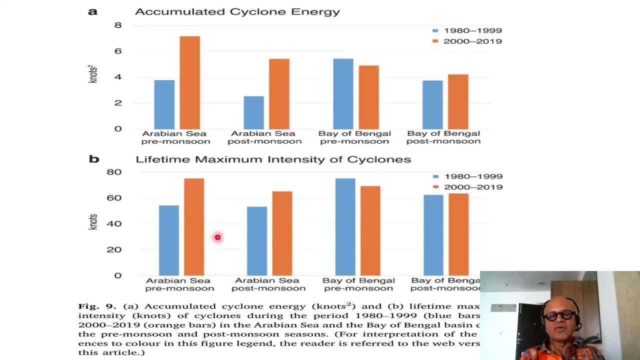 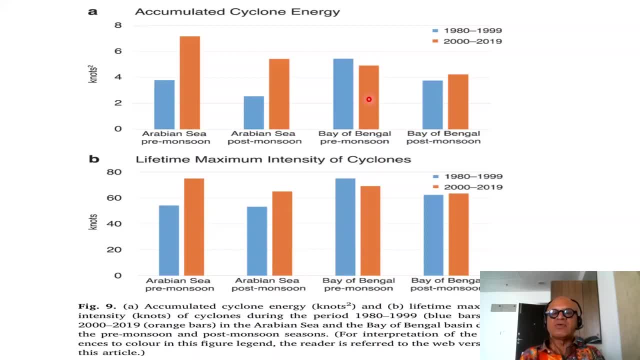 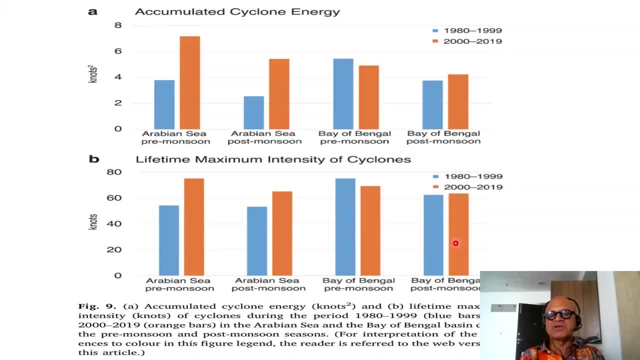 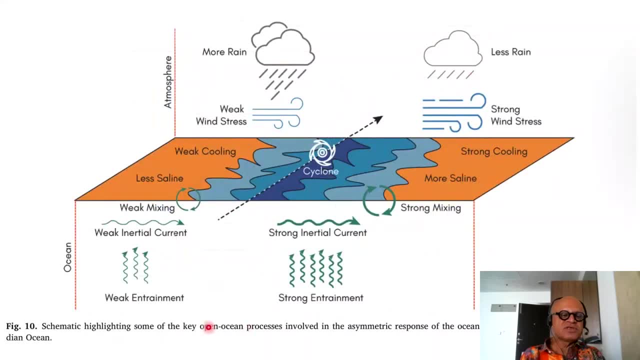 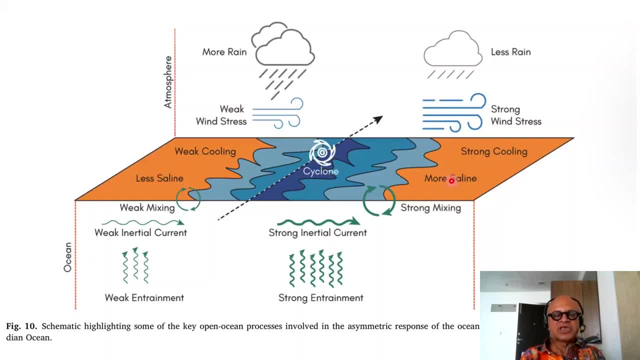 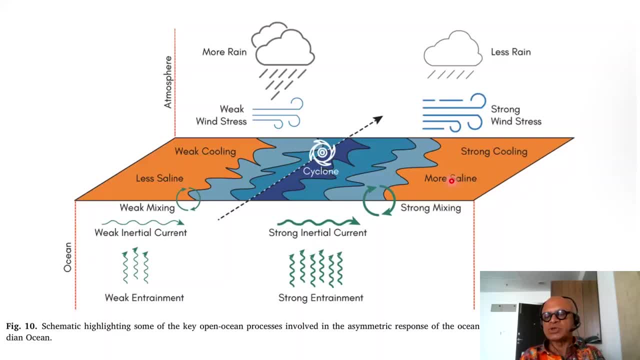 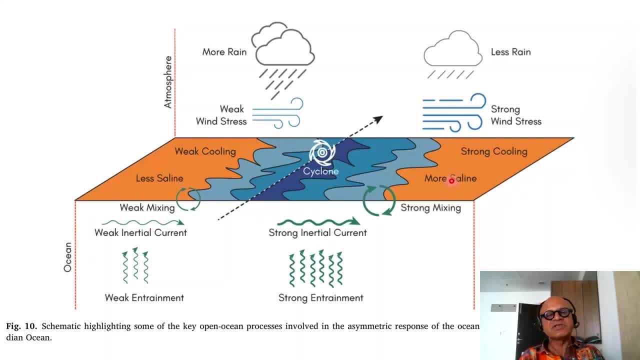 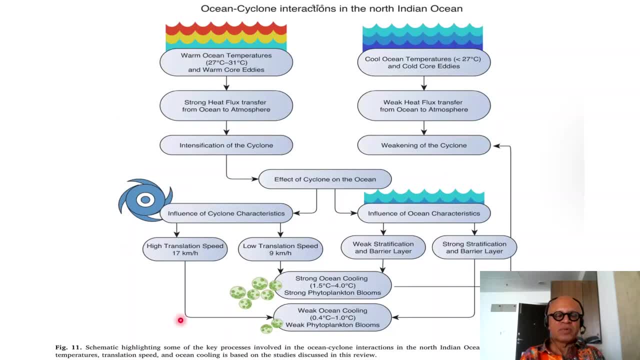 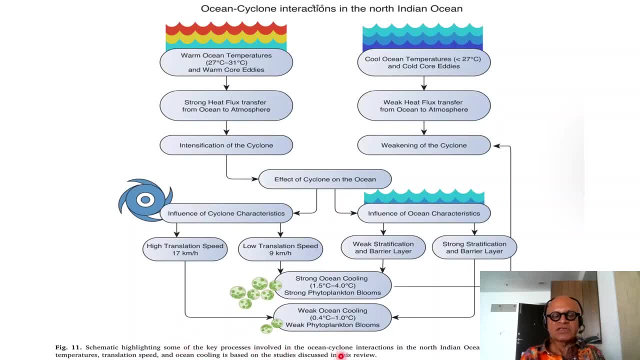 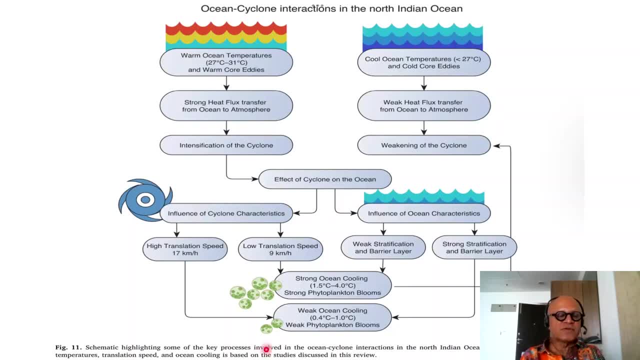 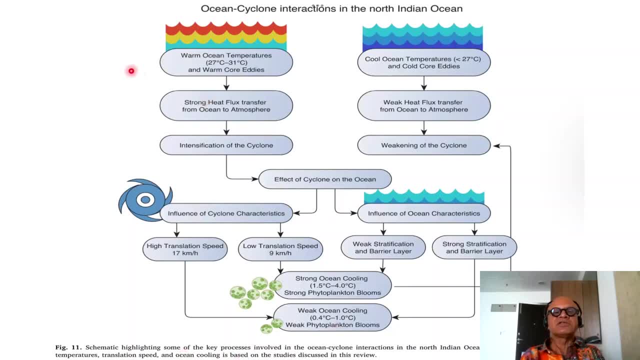 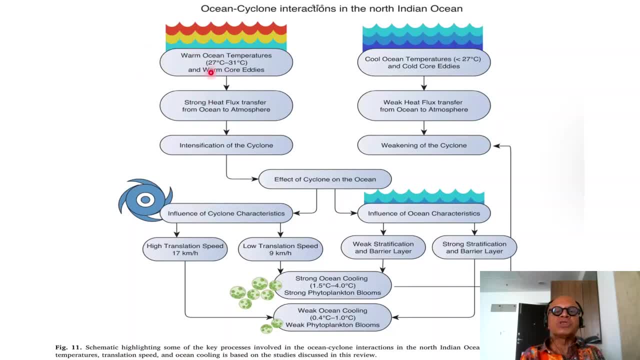 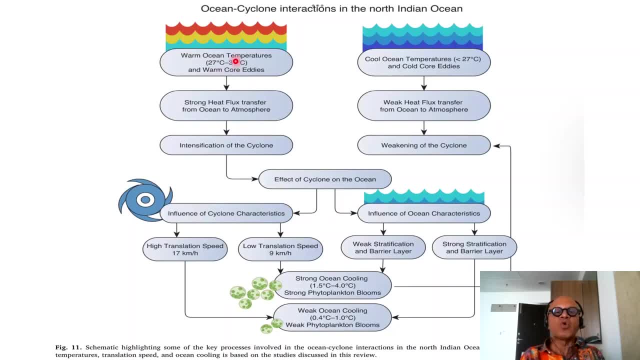 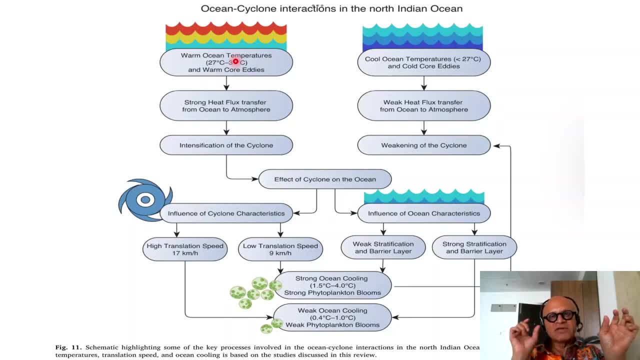 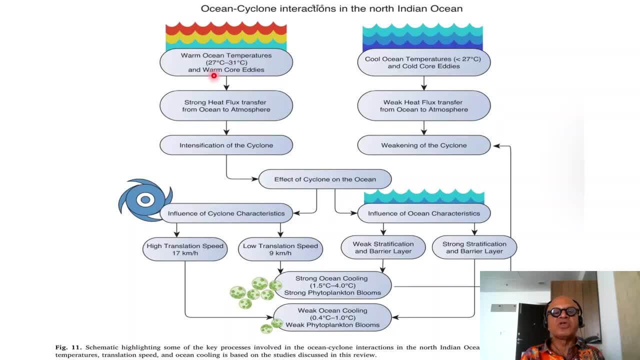 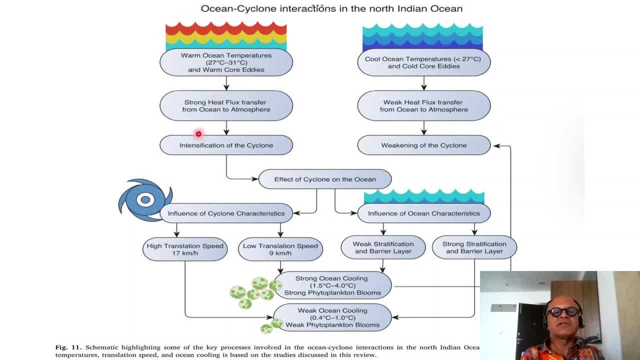 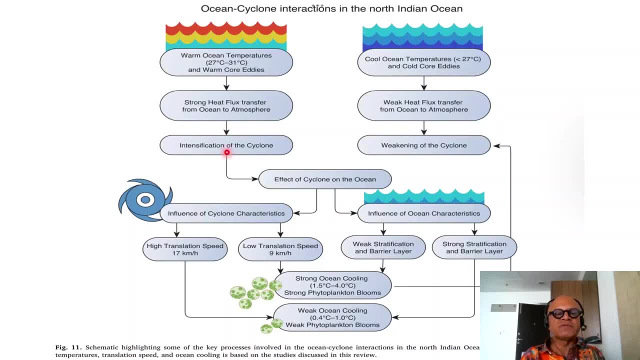 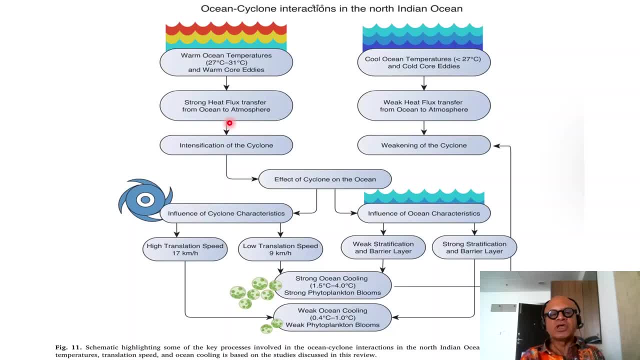 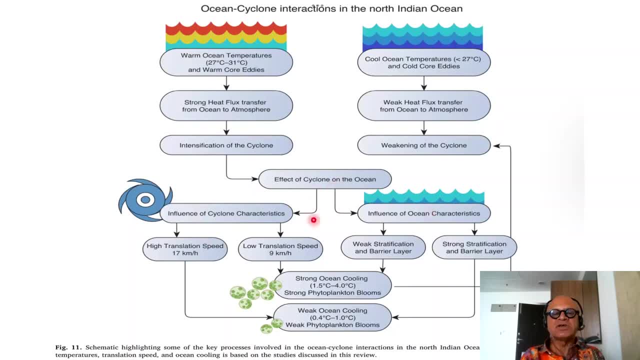 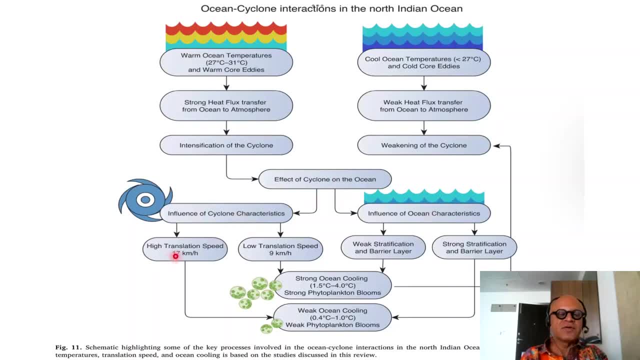 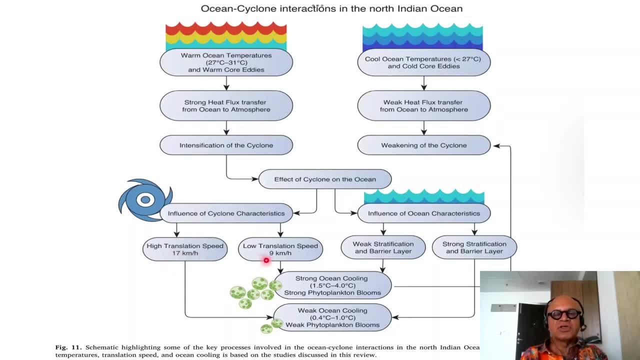 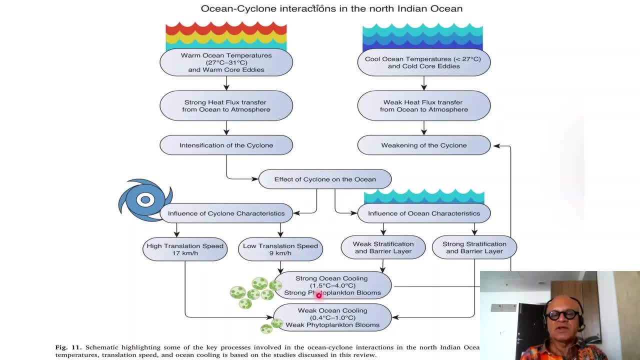 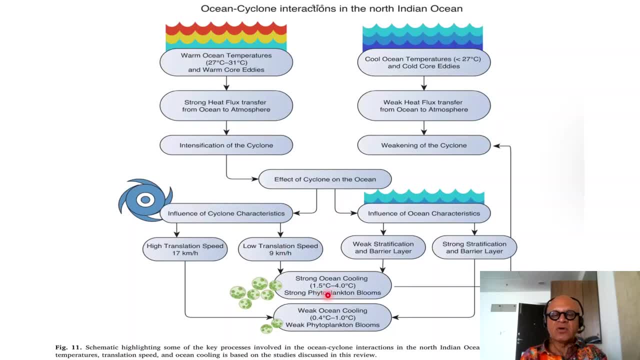 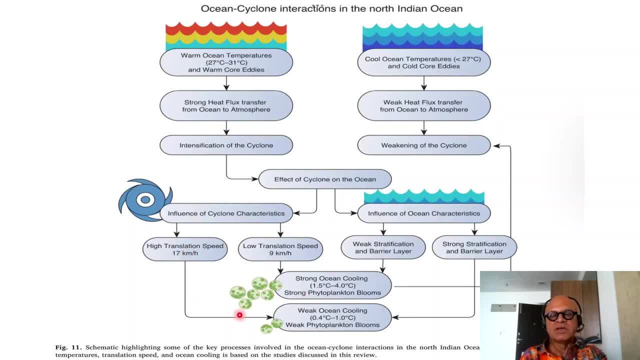 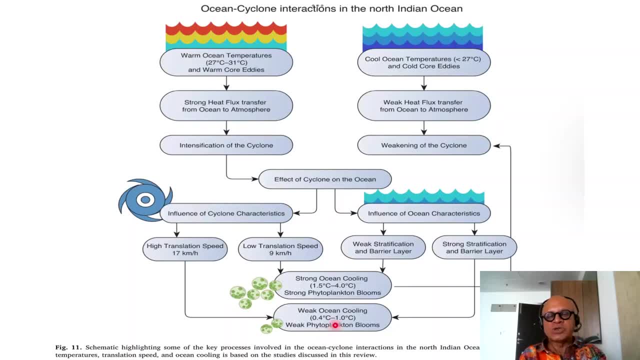 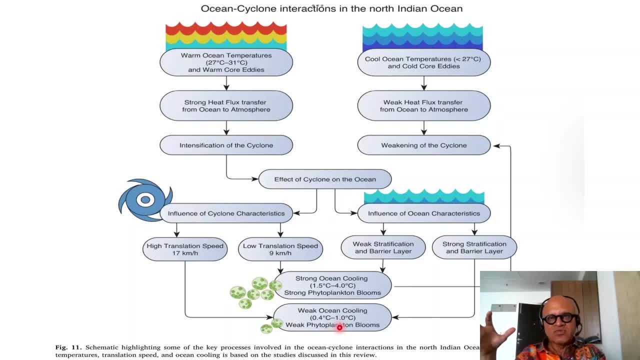 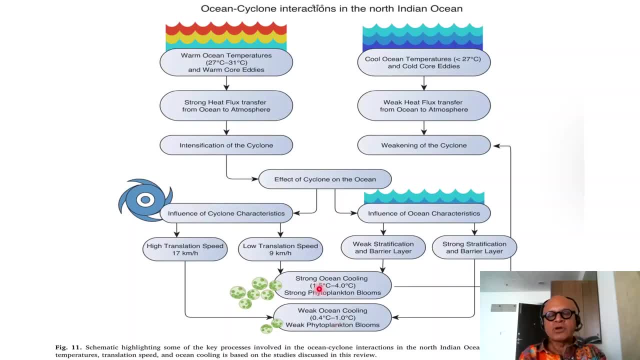 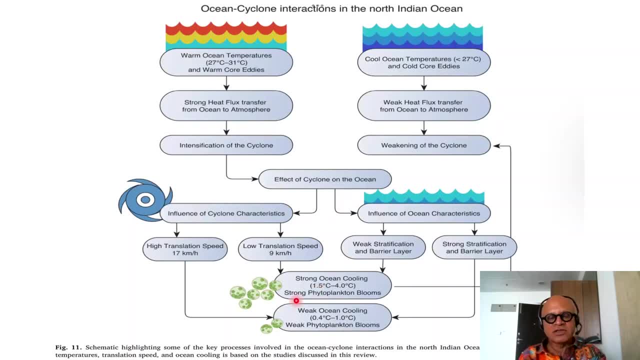 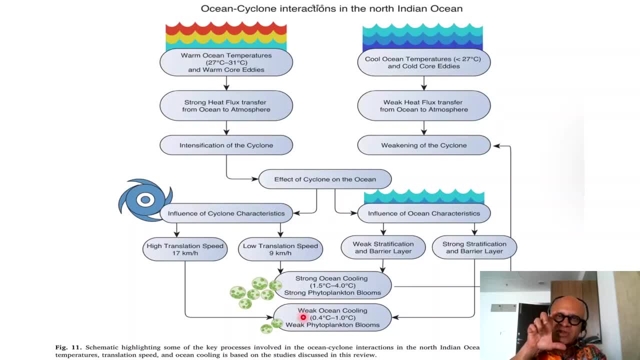 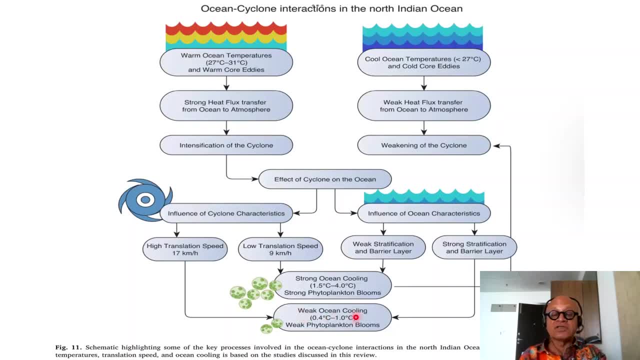 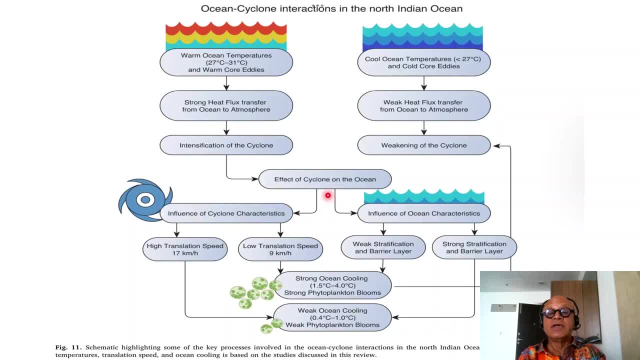 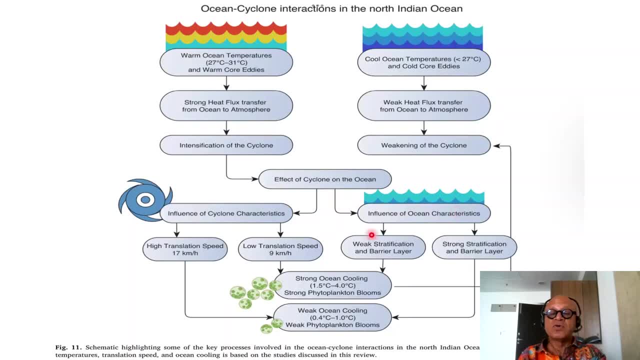 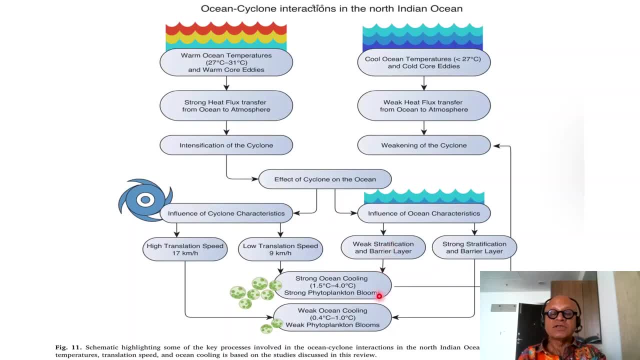 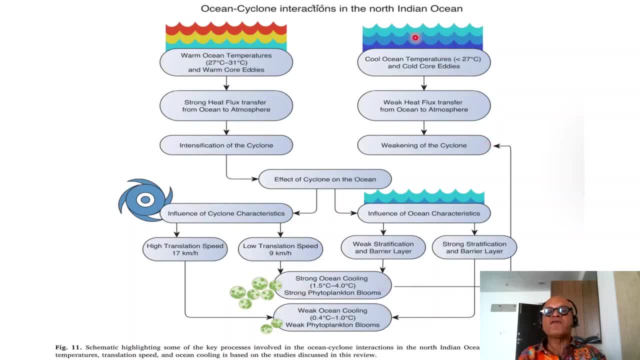 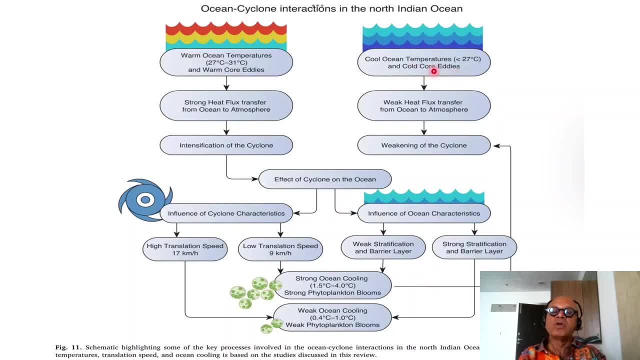 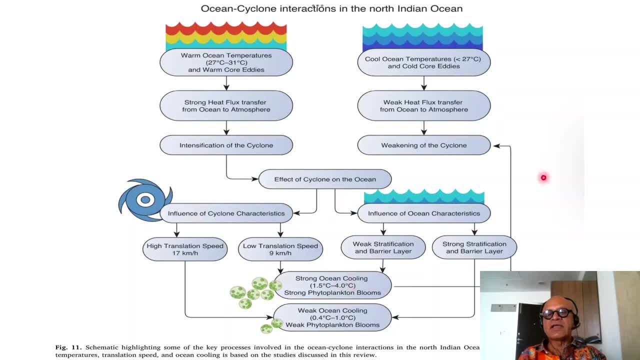 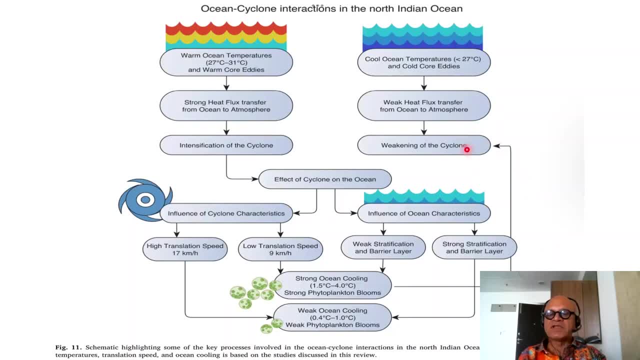 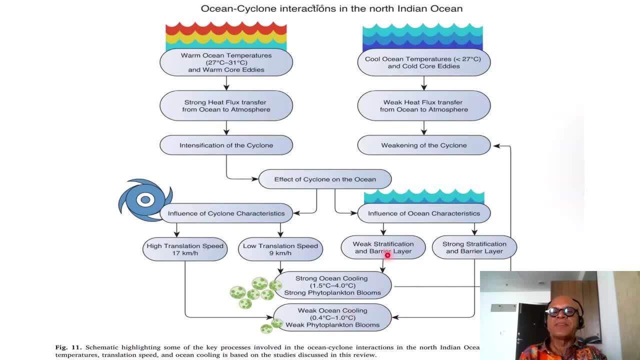 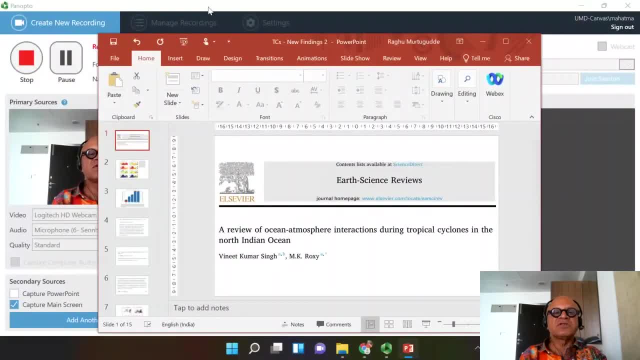 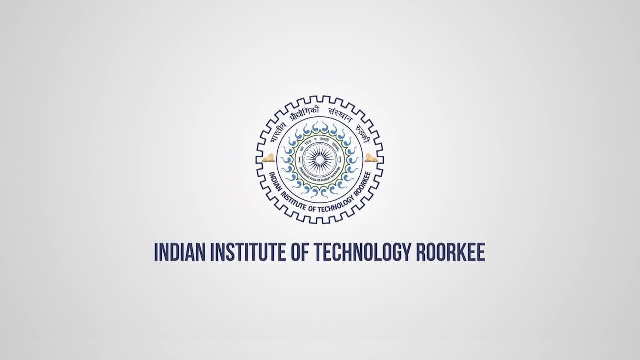 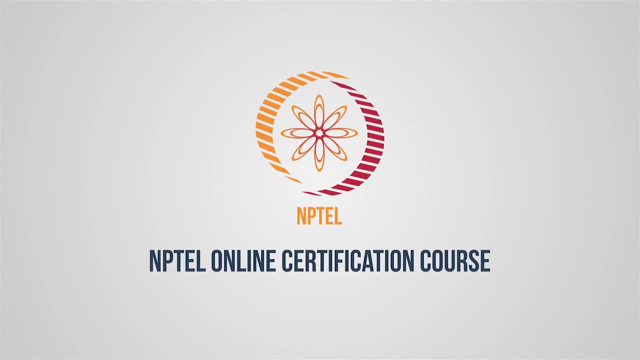 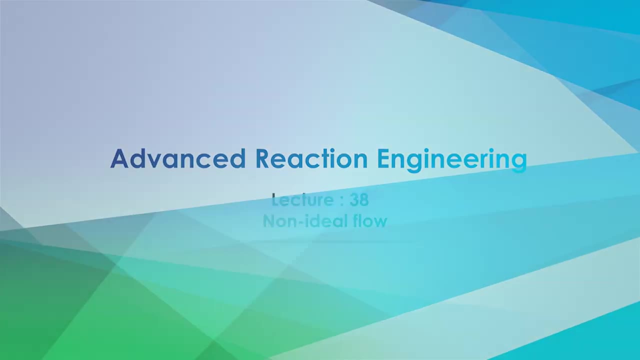 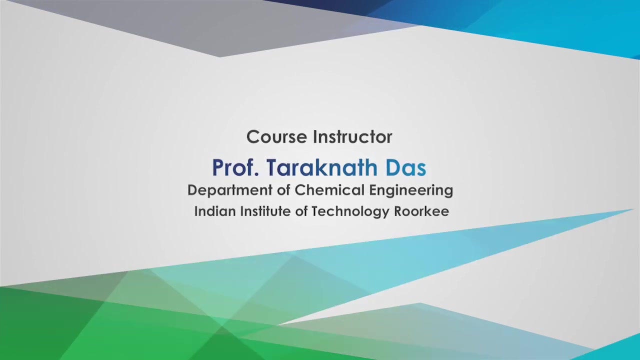 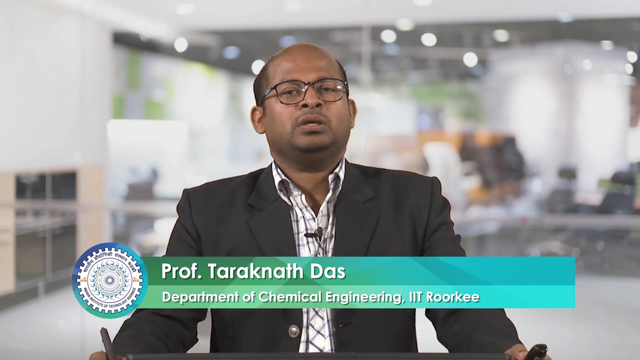 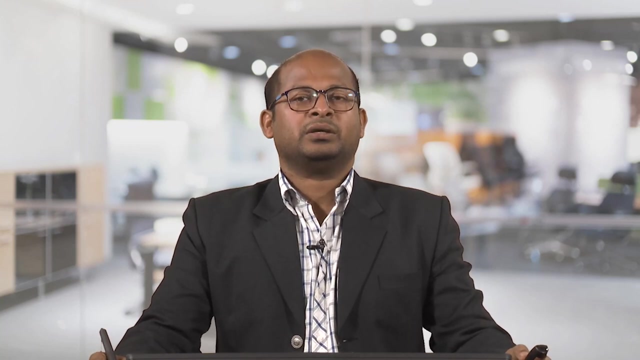 So welcome to the course Advanced Reaction Engineering. Today we will discuss about non-ideal flow. If we want to conduct any reaction, so then we have to choose the reactant, So we have to fix the reactions, and after that we have to choose any reactor. So there.